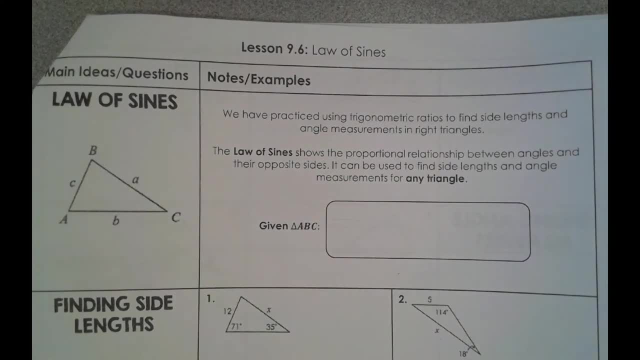 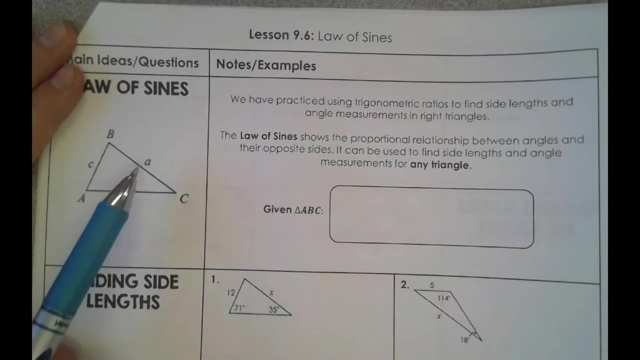 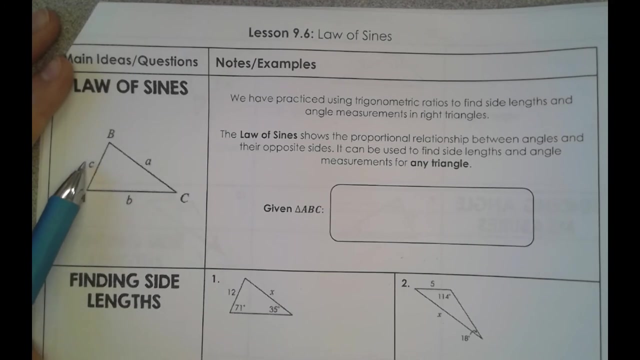 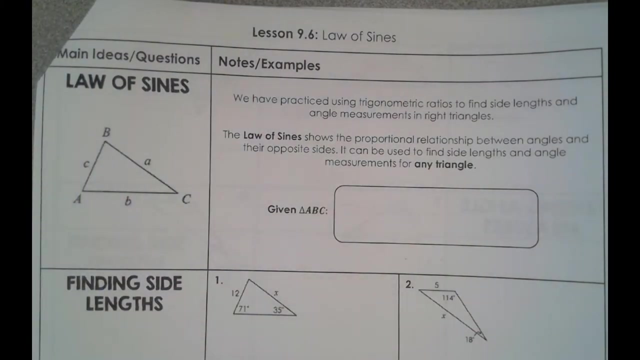 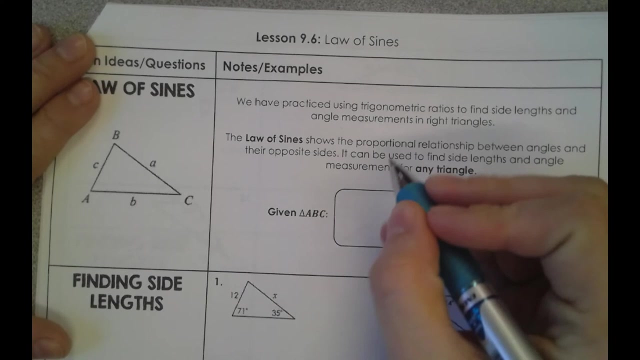 And so here is kind of a formula, not really a formula, but something like that. So notice how in this triangle the angles are marked with a capital letter And the side that is across from them is in the lowercase letter. So law of signs says that if I take sine of any of those three angles, so let's say sine of A. 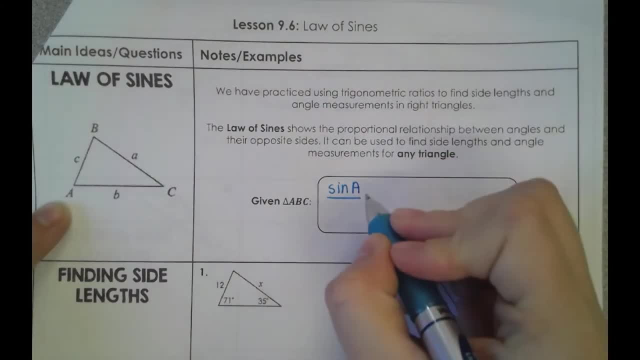 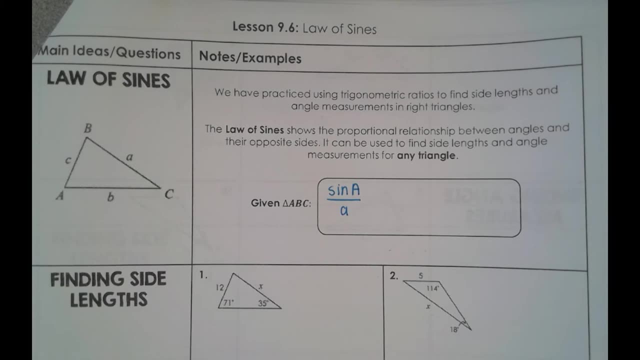 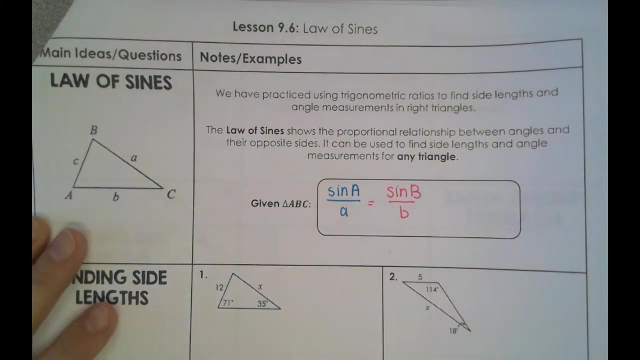 and we divide it by little a, So the side that is across from it kind of like, it makes like a proportion type thing That is equal to all of the other pairs. So that's equal to sine of B over little b, which is equal to sine of C. 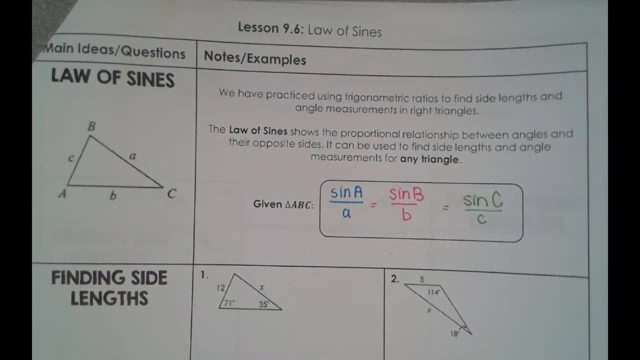 So that's equal to sine of B over little c. So with these we don't label opposite, adjacent. We don't label any of that. We're just taking sine of some angle measure and dividing it by the side length that's across from it. 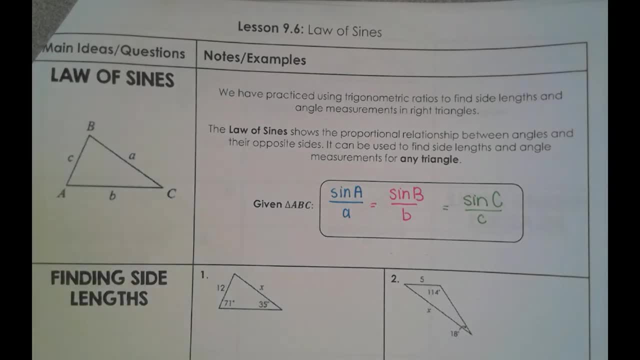 It's just kind of like a proportional thing that works within the triangles. So you have to have like a pair, You have to have an angle, You have to have an angle and the side length across from it for it to work, And then another angle across from your missing side. 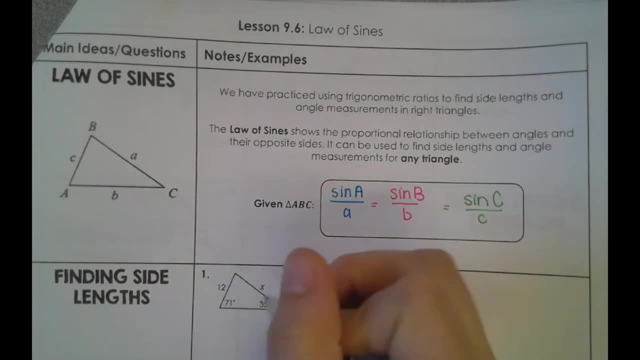 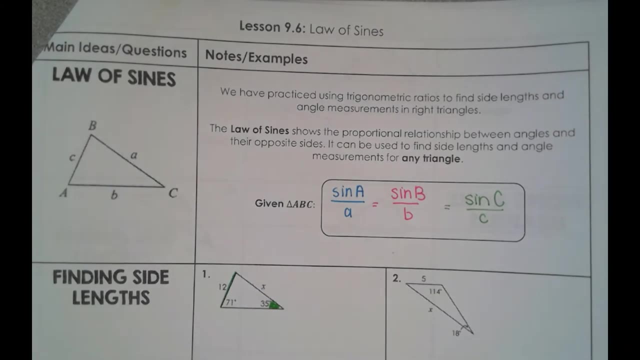 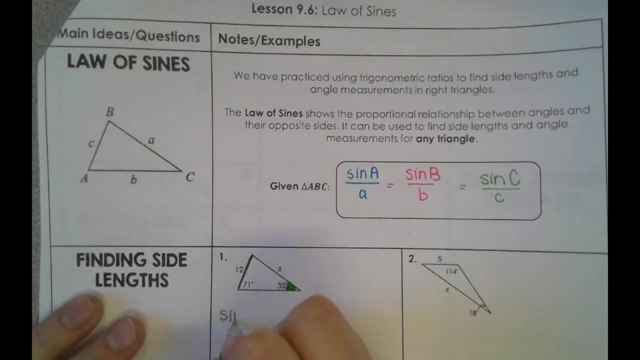 So if we look here at number one, notice I have angle 35 and I have the side across from it. Those are kind of a pair, Doesn't matter which one you call A, B or C, It doesn't matter. So we could say that sine of 35.. 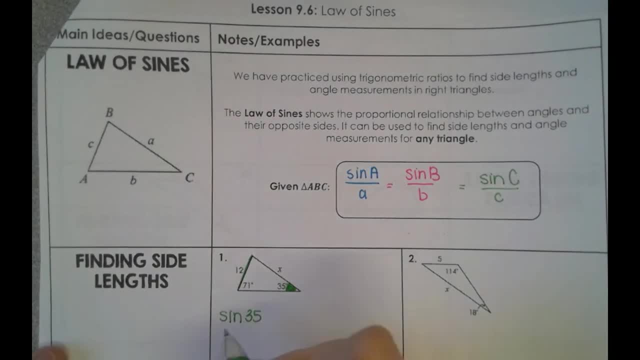 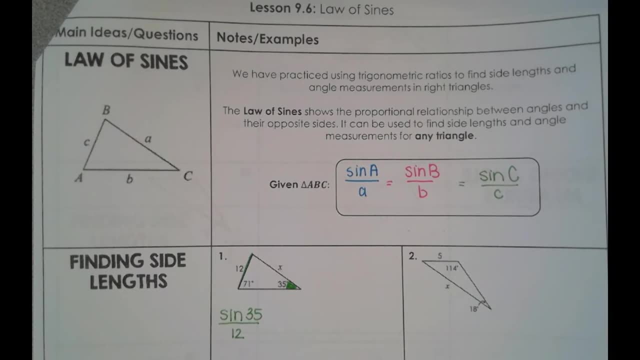 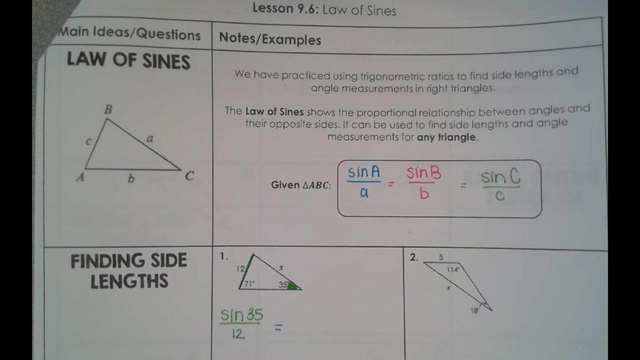 So it's always sine of your angle Divided by the side that's across from it, So 12.. That's equal to, And then I can pick another pair. We don't have to have all three pairs, We only need two pairs. 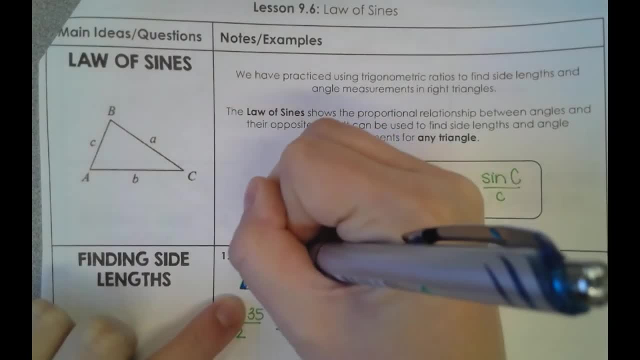 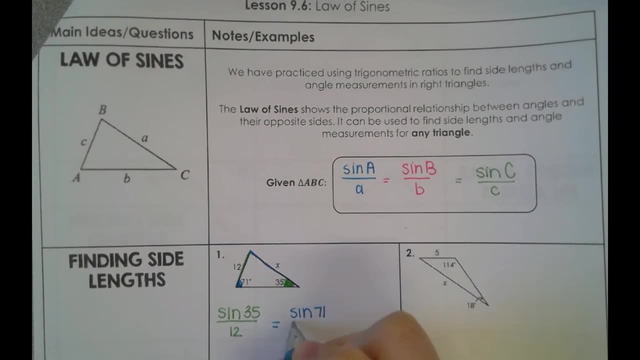 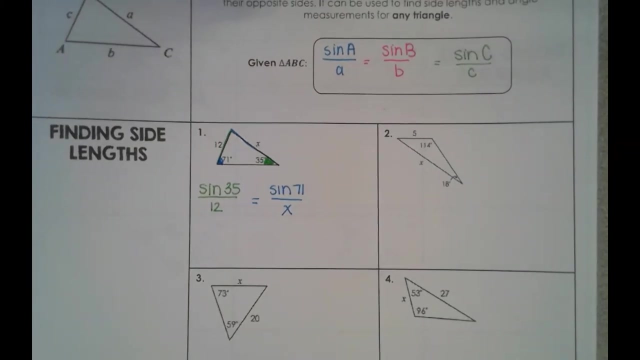 So notice how this 71 degrees is across from X. So sine of 71 over X. So you've got to make a pair. You have to have an angle and the side across from it. Now, luckily, if we have two angles in a triangle, can't we find the third one easily, right? 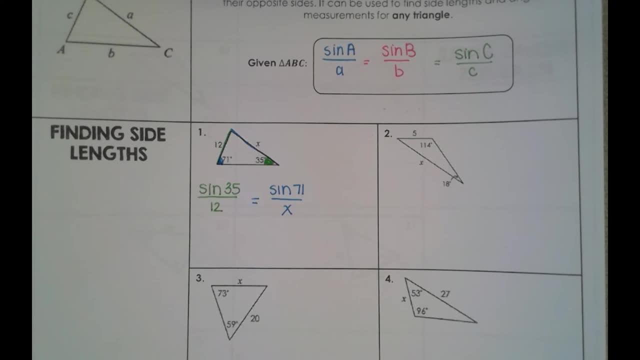 So if we have two, we really have all of them. They may not all be labeled, but it's really easy to find them because you just subtract from 180. And so that's really not usually a problem. Um, But you've got to make sure you stick the angle with the correct side. 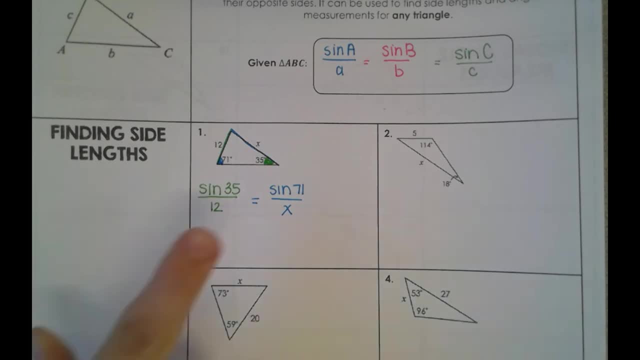 It has to be the one that's across from it. So now we can cross, multiply, So X sine of 35. So we multiply those two Equals 12 sine of 71. And then to get X by itself, We divide both sides by sine of 35.. 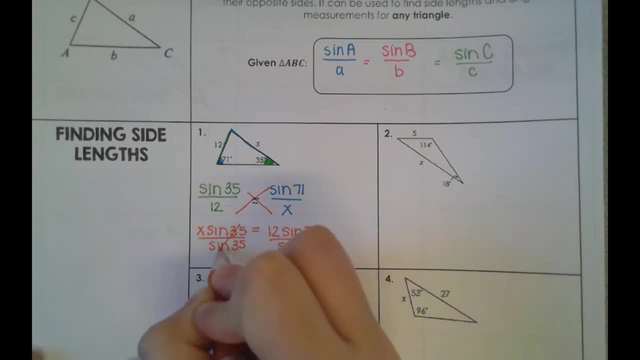 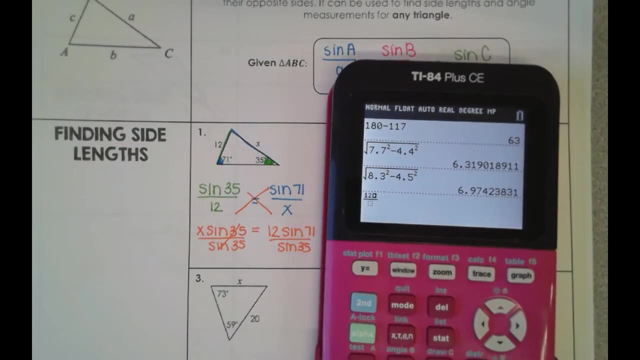 And you can do that all in one step on your calculator. 12 sine of 71 divided by sine of 35.. Make sure your calculator is in degree mode. Some of you found yesterday You were getting some really weird answers because your calculator was in radians. 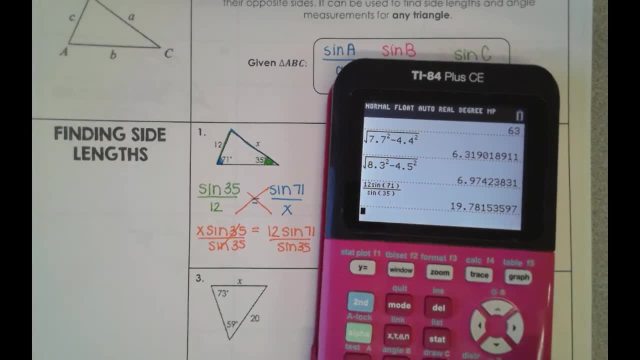 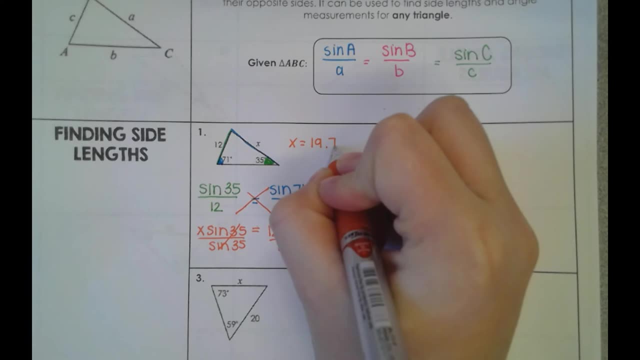 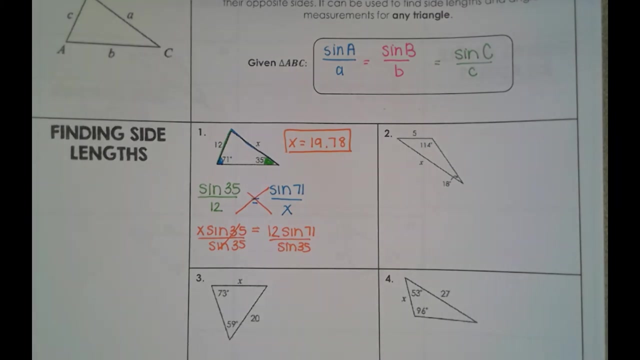 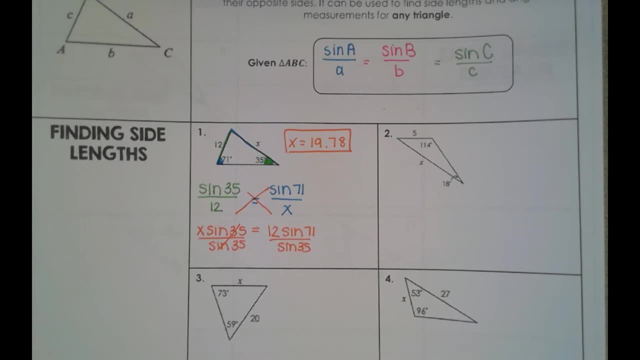 19.78.. 19.78.. If you look at my trash can, there's like a bunch of these little. Did you say it needs to be in radian? No, it needs to be in degree. Did I say radian? 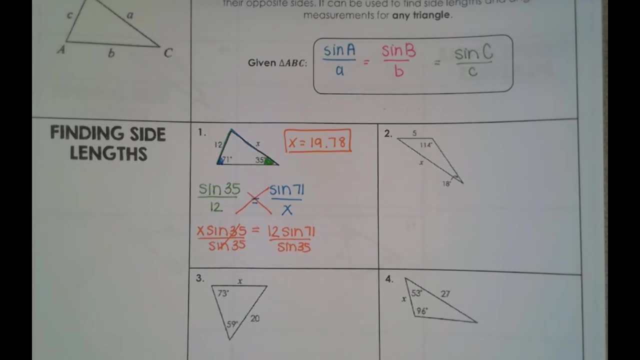 It needs to be in degree. Sorry, My bad. They were better yesterday, They were better yesterday And now they're back again. All right. So number two: let's look for our angle side pairs. So this 18 degrees. I've got that one. 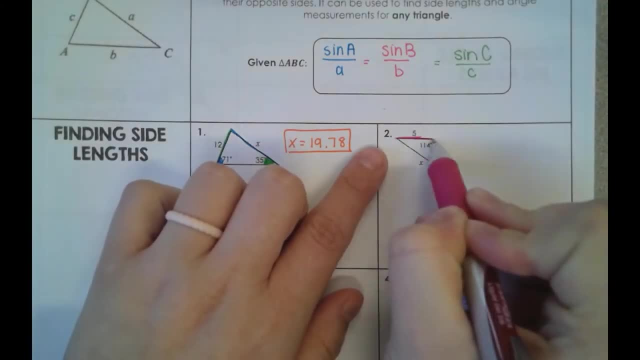 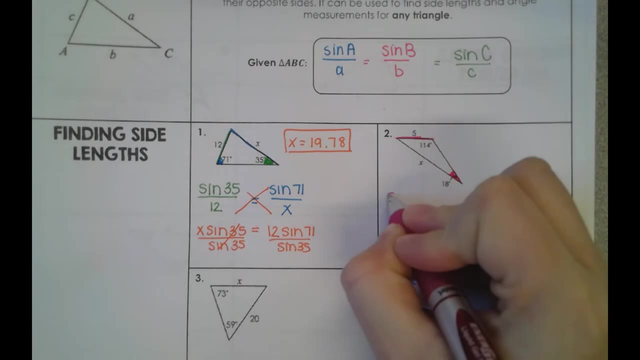 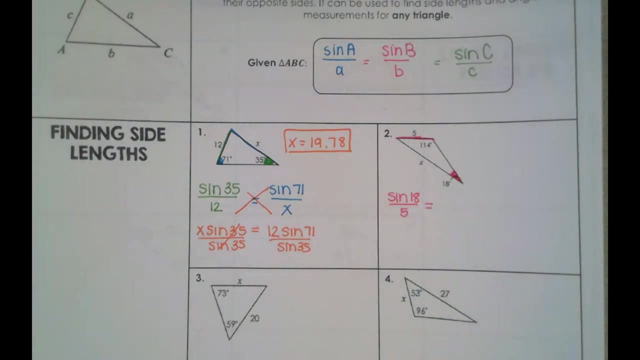 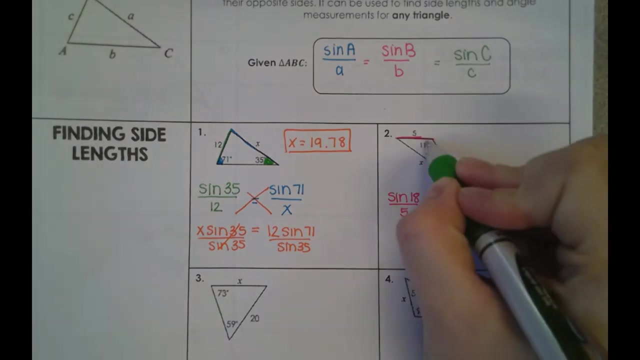 And if I look across the triangle, that matches up with the side length of five. So we can say sine of 18.. And then we have our false side. How many times in the length of the triangle is 1,, 14, over 5 equals? and then we do have. 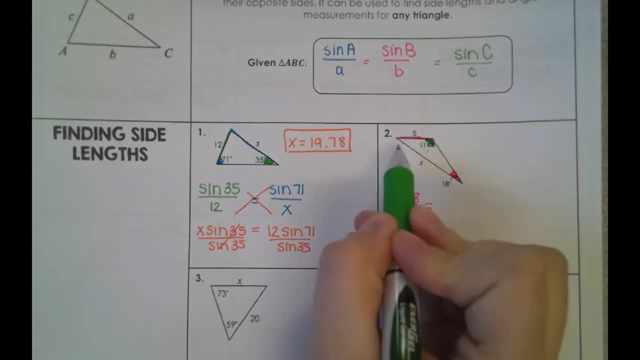 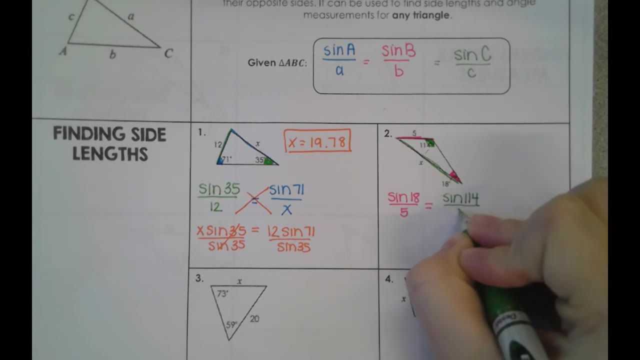 this 114, across the triangle is X. So sine of 114 over X. So that's the. that's the problem, And if I go across the triangle I end up getting x. So I want to make sure that I'm getting this 2 times. 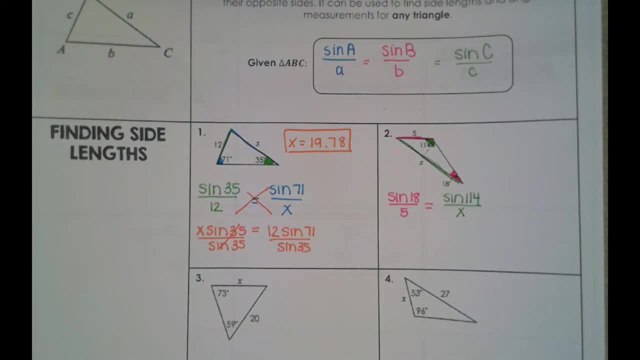 So I want to make sure that I'm getting this 2 times. I want the same thing, And then I want to make sure I get my right side, so It's a right side, And then I want the opposite side- Right side. 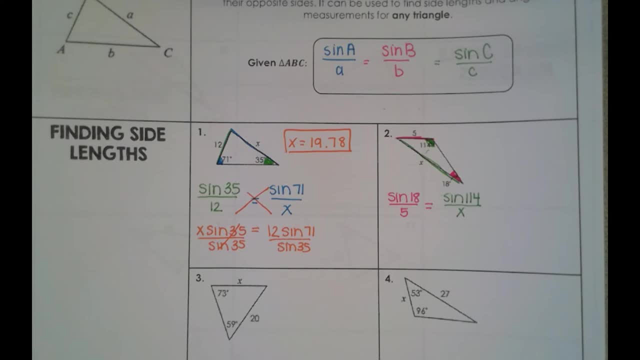 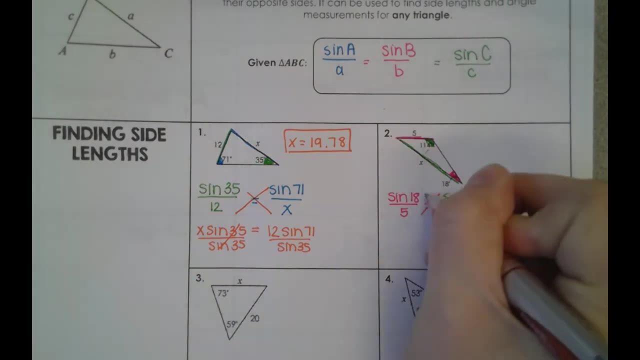 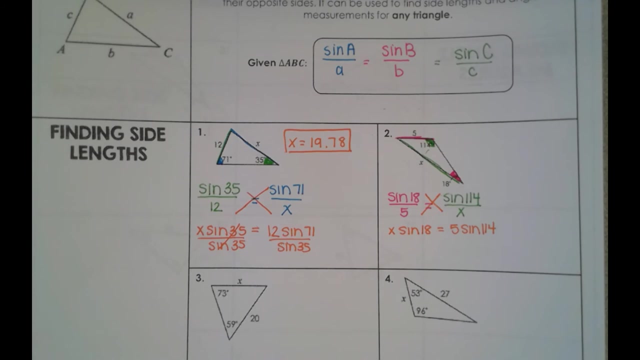 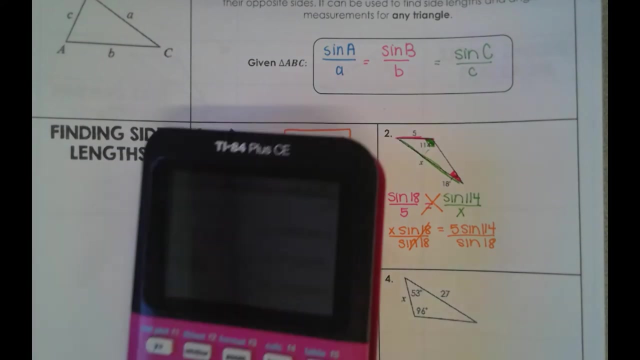 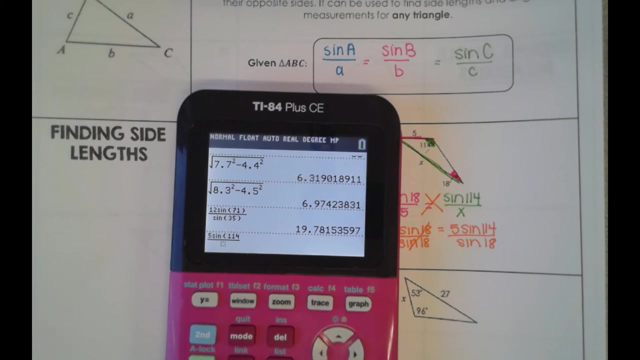 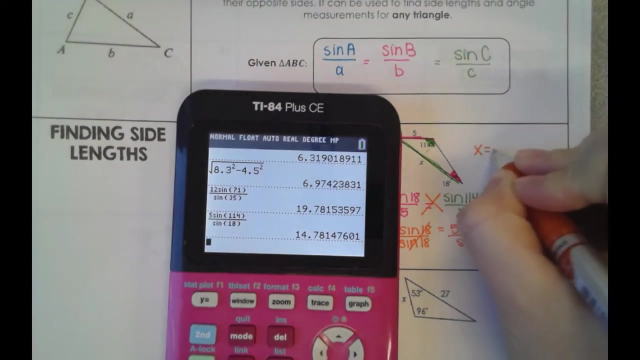 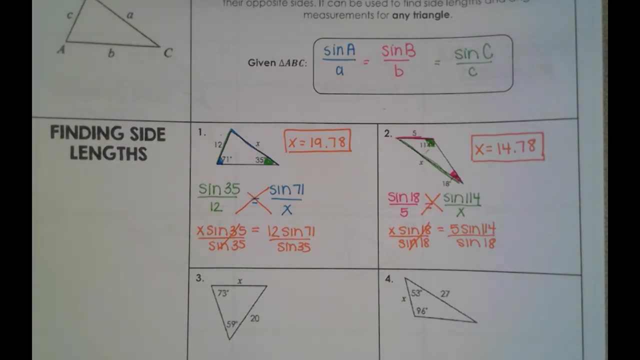 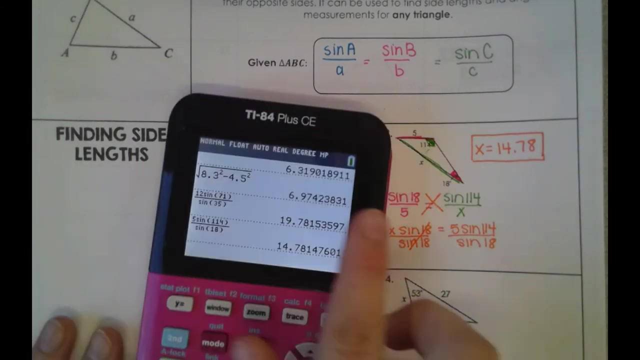 Right side, Right side. So when we cross multiply we get X sine of 18 equals 5 sine of 114.. And then if we divide both sides by sine of 18. We get X equals 14.78.. Does your calculator say degree? 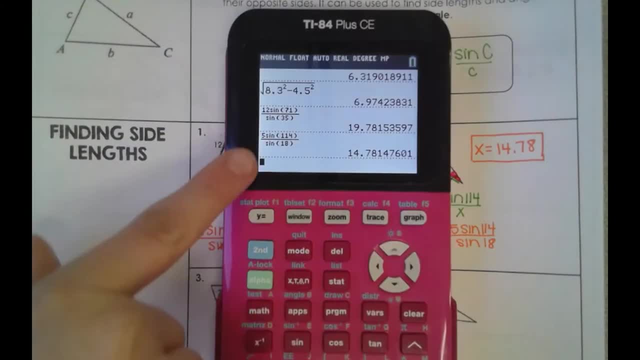 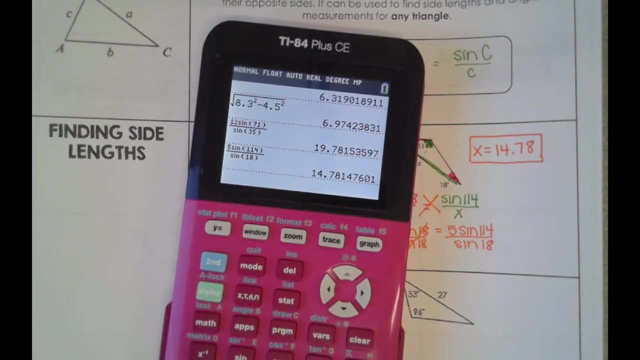 Yes, And you did. did you type it in like this: 5. 5. Okay, If you are just doing, if you're just doing the divided, make sure, yeah, you got to close your parentheses, Because it it'll put that rest of that within the parentheses. 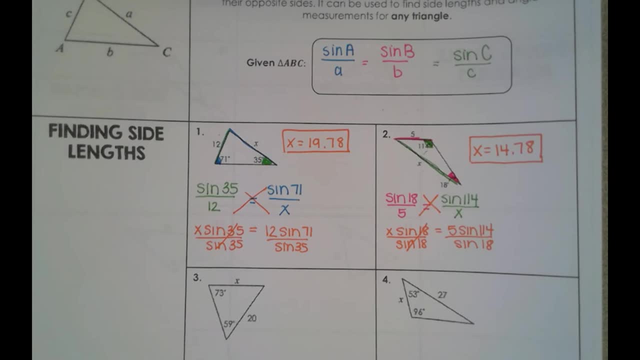 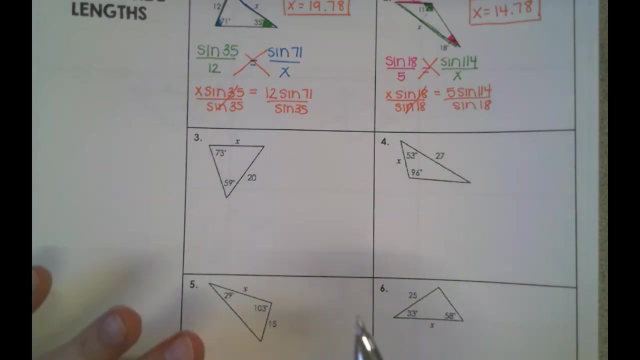 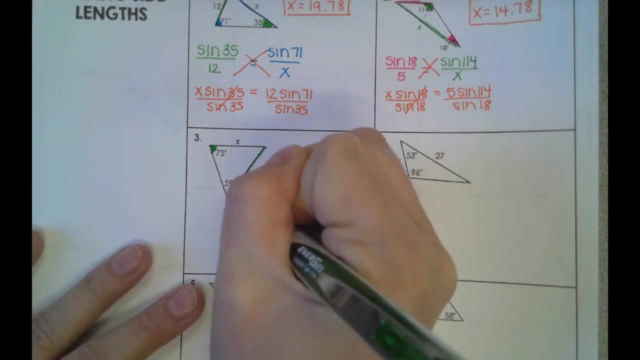 Yep, Okay, Any questions? All right, Let's look at number three. There we go, All right. So let's pick out our pairs. So let's see This: 73 degrees pairs with the side length of 20.. 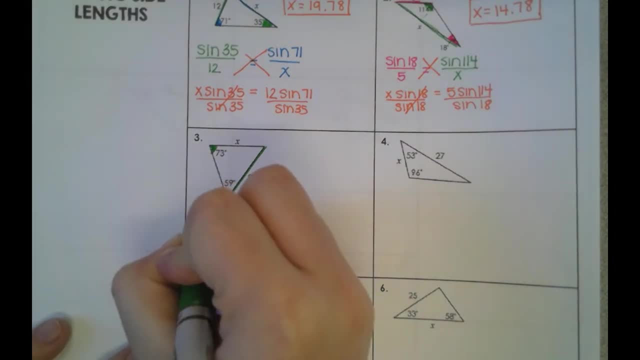 Because they're a cross. So we can say that sine of 73 over 20 equals. And then I need this 59 degree angle because it pairs with the X, what I'm trying to find. So sine of 59 over X. 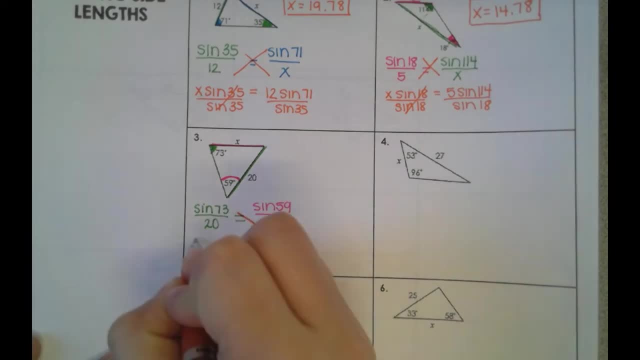 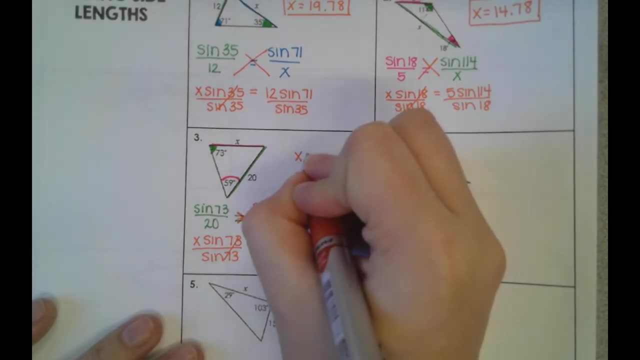 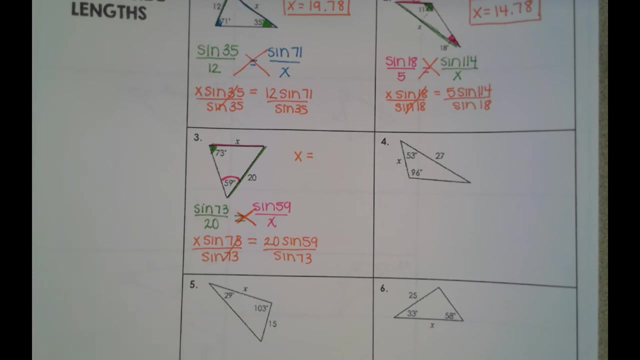 Then I'll cross: multiply X sine of 73 equals 20 sine of 59.. Okay, And then divide by sine of 73.. Okay, And you should get seven, Okay, Okay, Okay, Okay, So we have 15.93.. 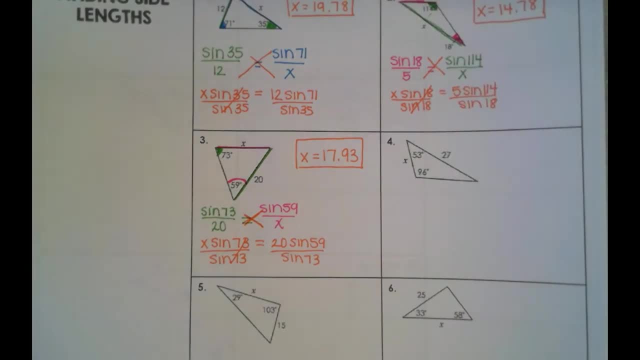 Number four. Let's see This: 96 degrees will pair up up with the 27. So sine of 96 over 27.. However, my other pair, I have to use this side length of x, so I need this angle. I don't have that angle, but we just said it's easy to find. So if we take 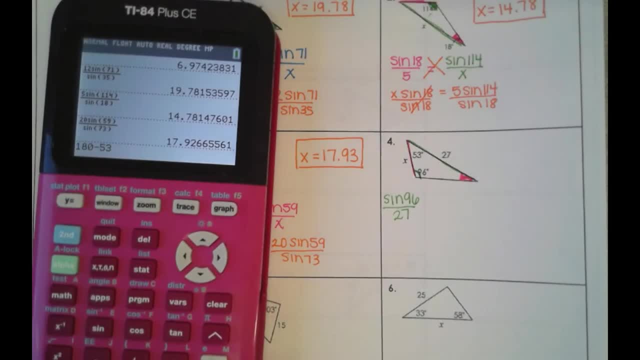 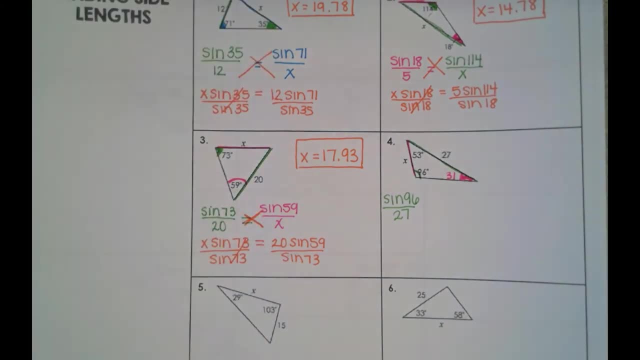 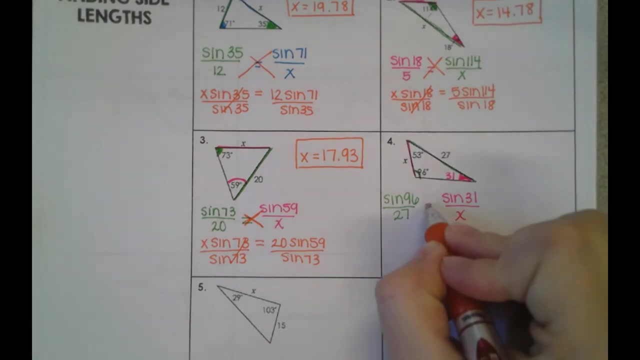 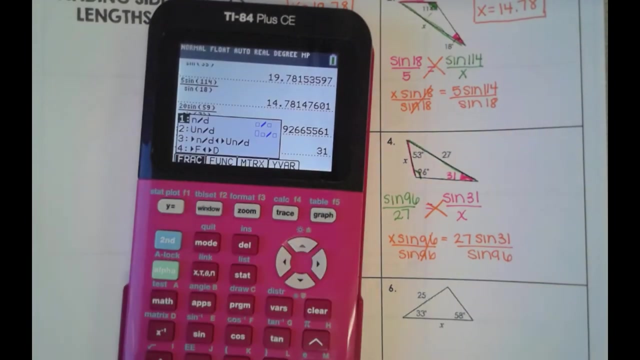 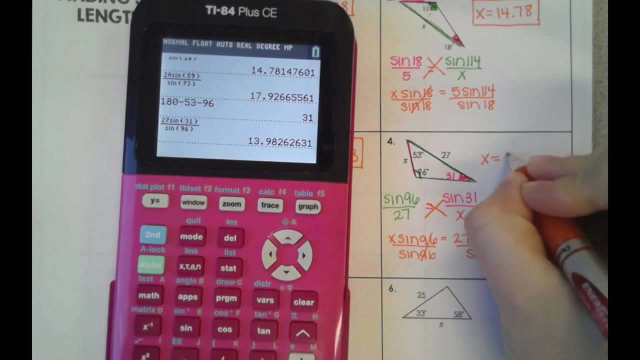 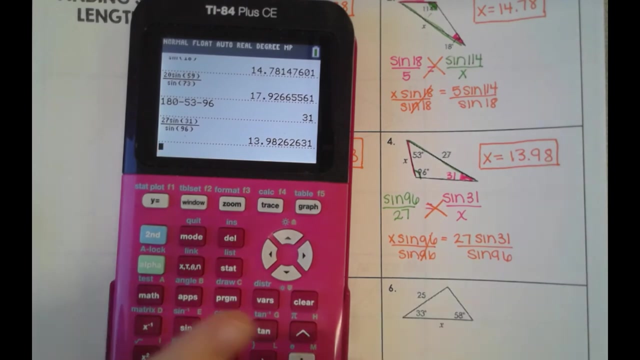 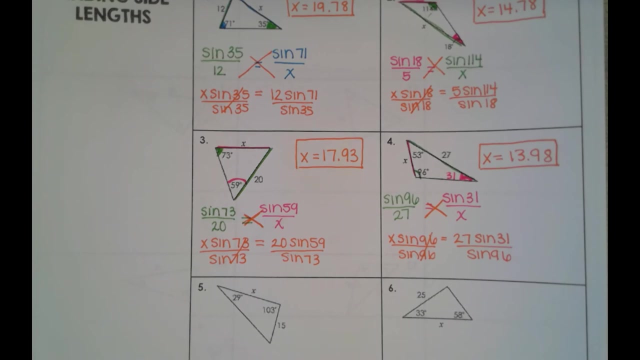 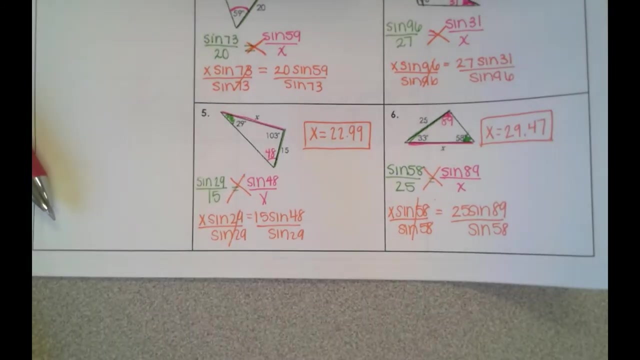 180 minus 53 minus 96, we know that angle is 31 degrees. So sine of 31 over x Cross multiply, Cross multiply X equals 13.98.. Try questions five and six. All right, so you should have got 23.. 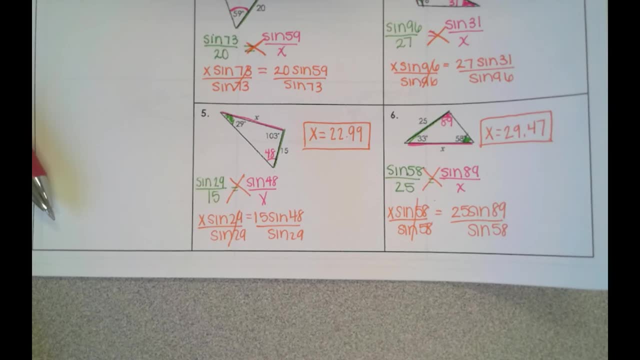 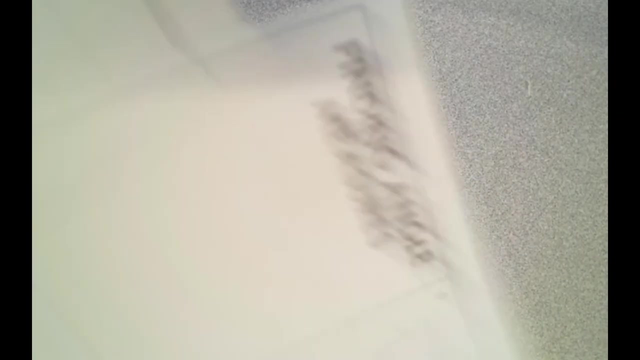 You could have wrote 23.. You could have wrote 23.. You could have wrote 23 or 22.99 on number five and 29.47 on number six. Are there any questions on these? Okay, let's get into looking at. oh, there's two more. 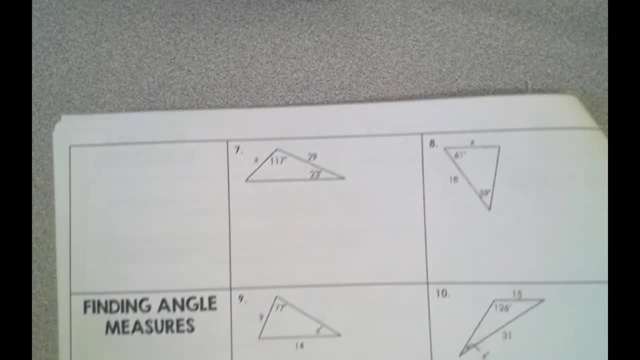 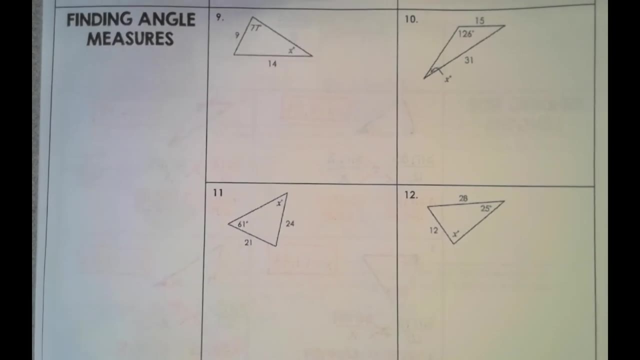 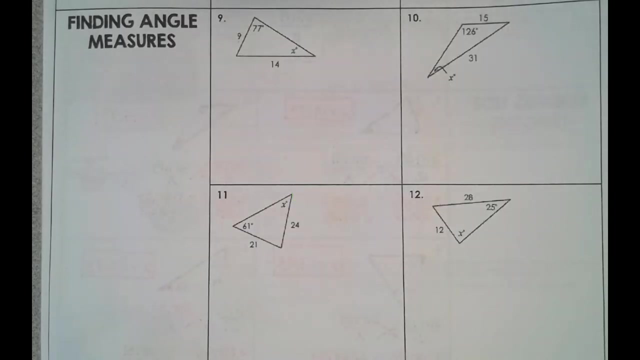 Let's see We'll just skip those, because you ought to get on those. All right, let's go down to number nine, where we're finding missing angle measures. Now, these kind of might need to make sure you're writing kind of small on these, because they do. 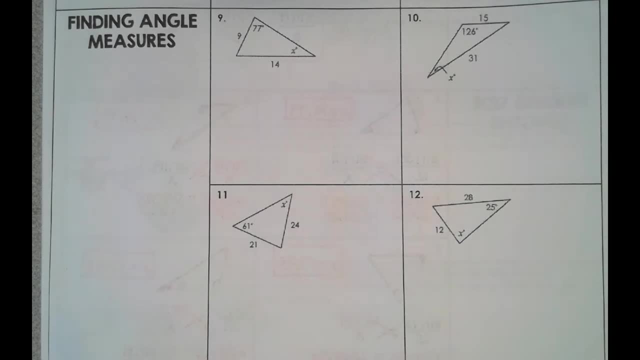 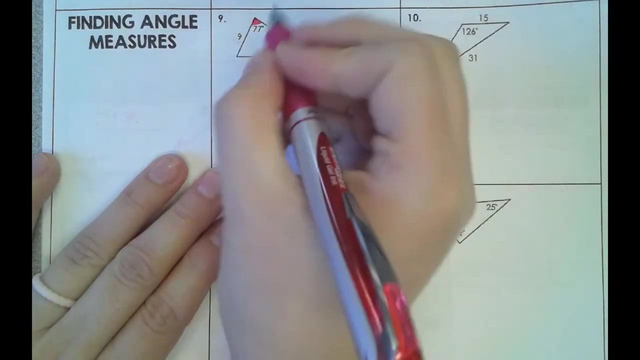 take a little more work on them. All right, so we start with same thing. We're going to set up our proportion, So get your angle side pairs. So, for example, the 77 degrees across the triangle is the side length of 14.. 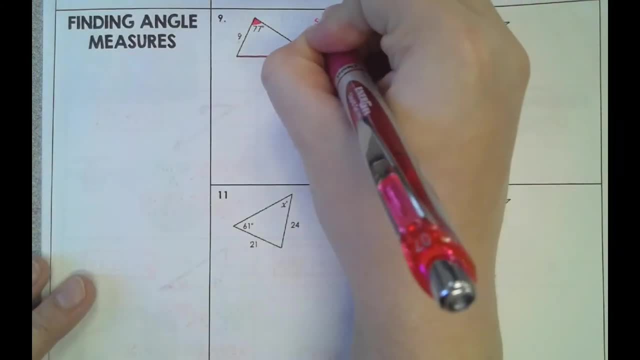 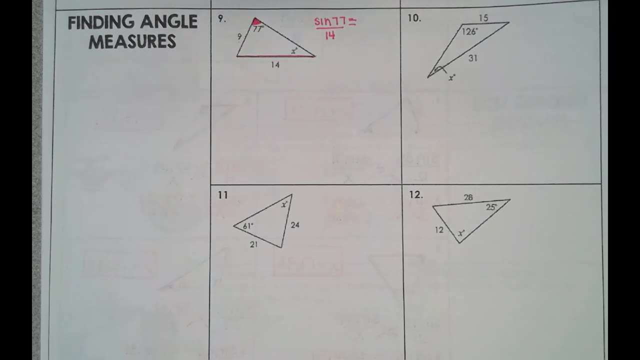 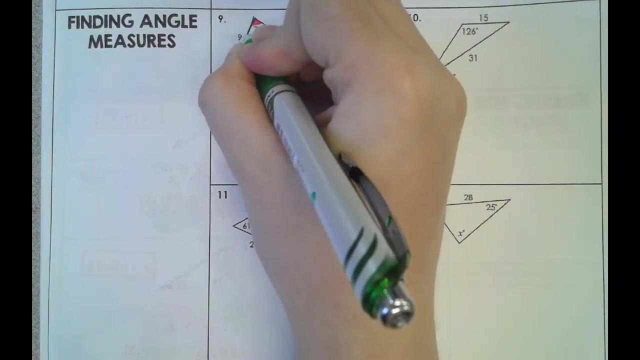 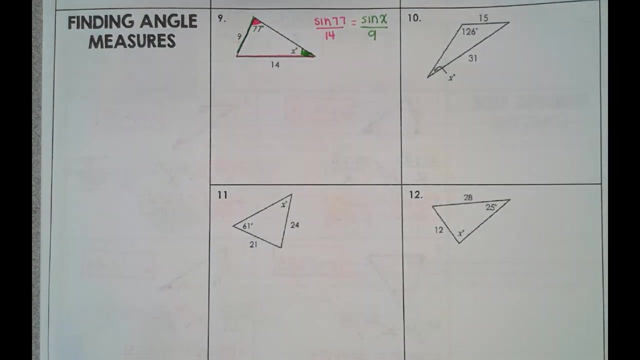 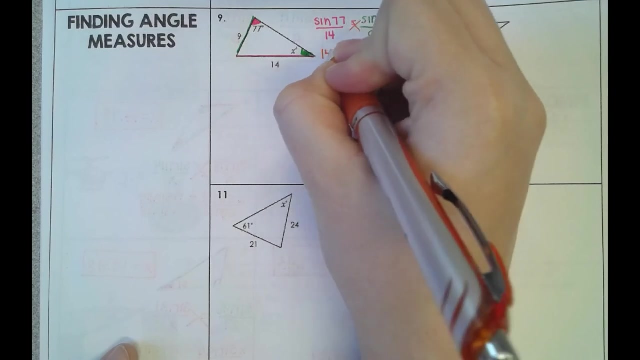 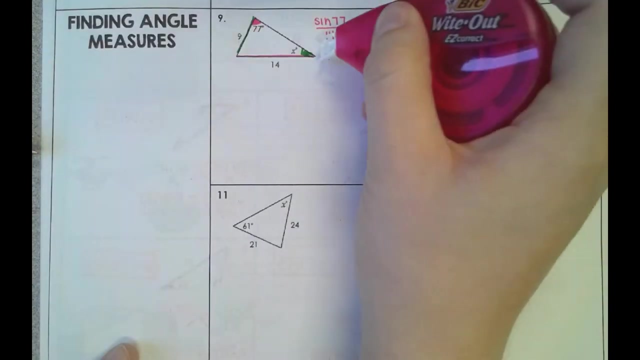 So I can say sine of 77 over 14 equals. and then my other pair, I use X and this nine. So sine of X Over nine. Now when I cross multiply we get 14 sine of X. Oh, let's see. 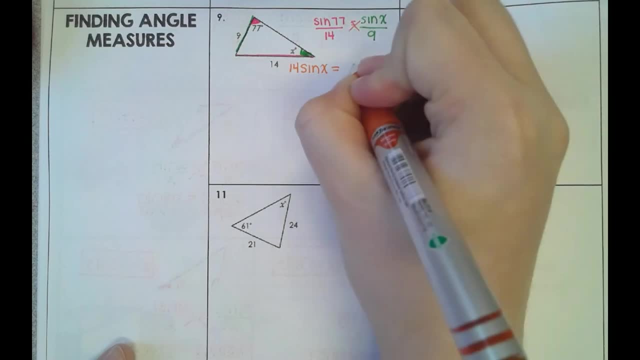 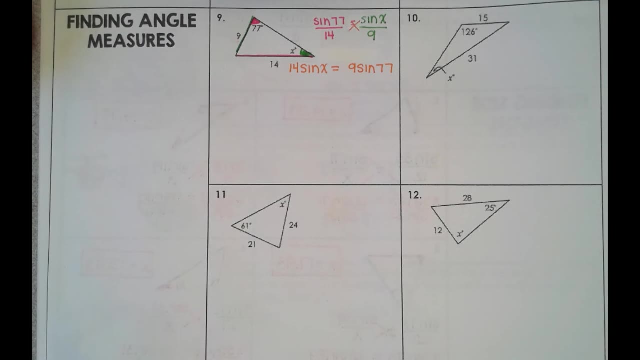 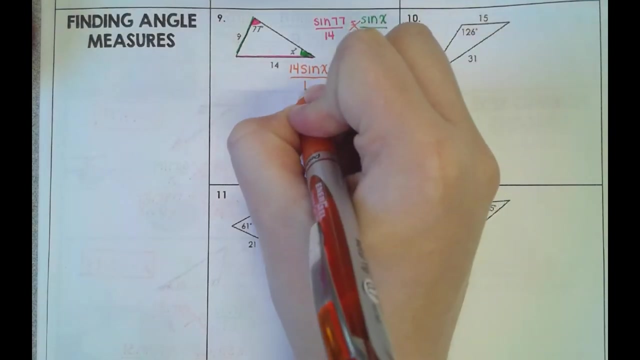 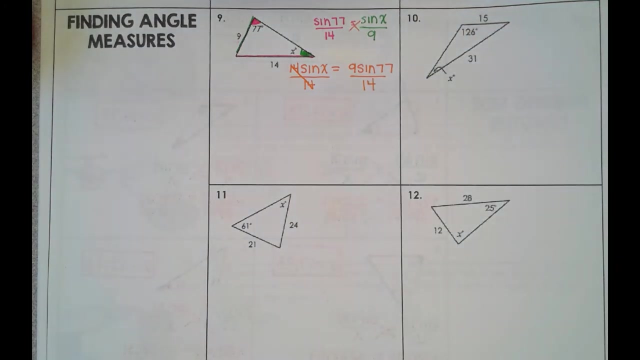 14. sine of X equals 9. Sine of 77. And then you need to divide both sides by 14. So if we divide by 14. Now you can go ahead and type that in this part over here and get a decimal. 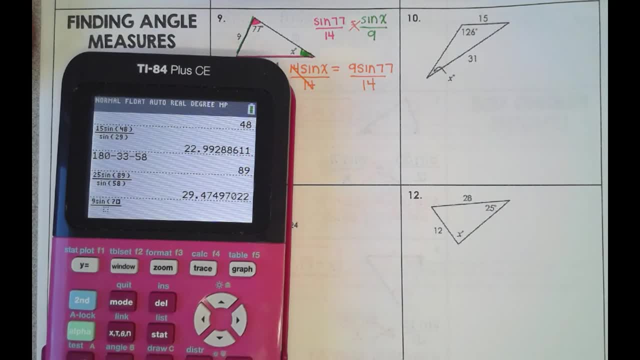 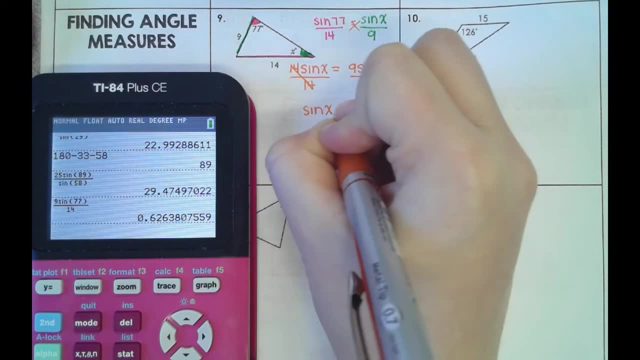 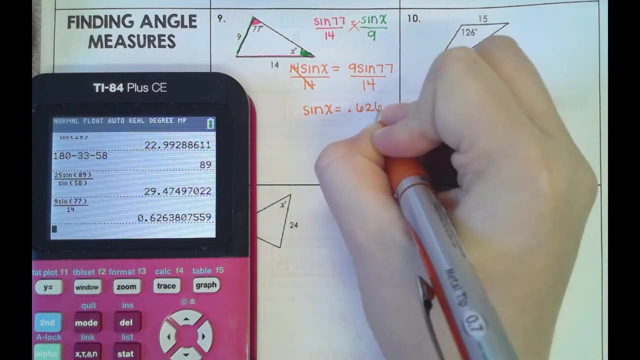 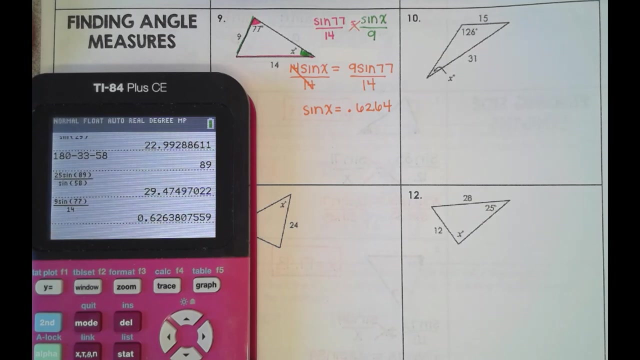 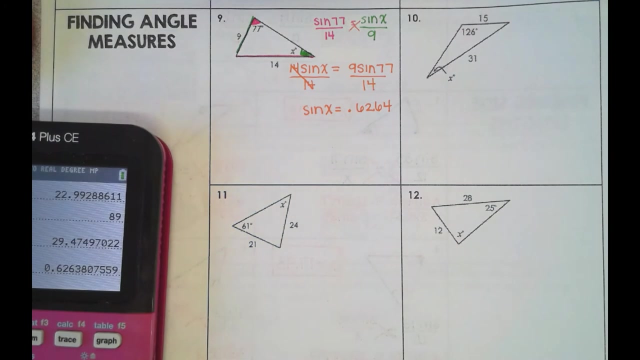 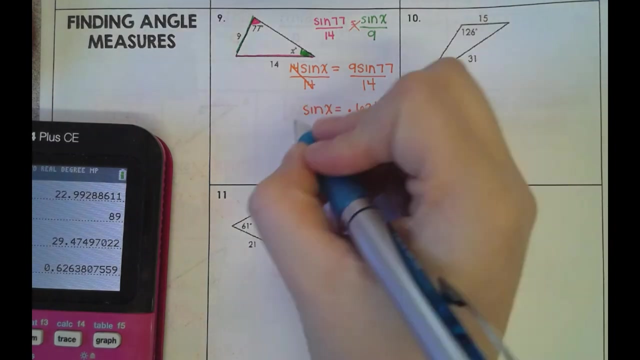 9, sine of 77 divided by 14.. But you need to go to at least 4 decimal places. So sine of X equals equals point six, two, six, four. but we still need X. so what do we do when we're missing the angle? how do we solve for that? do what we do, the inverse. so we do. 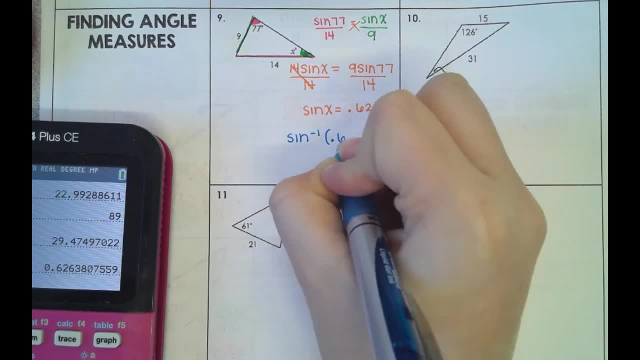 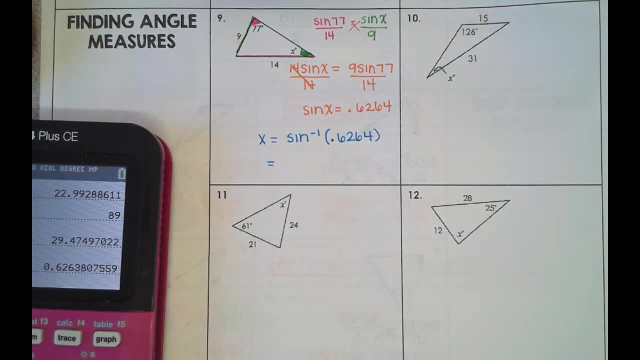 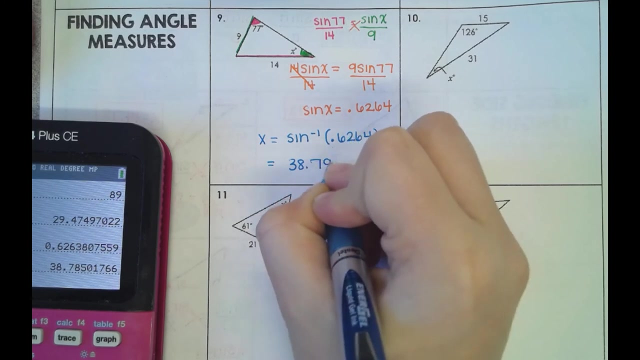 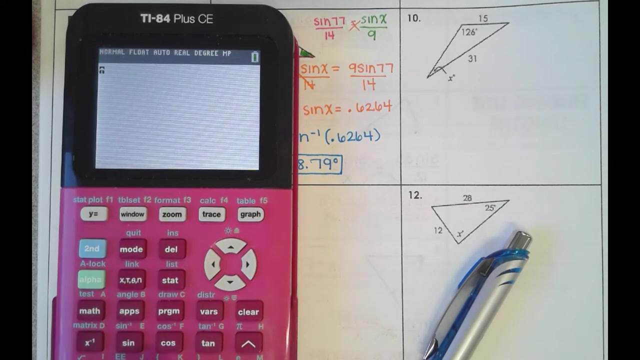 sine inverse of point six two six four. that's where you get second sign and you type in the point six two six four. you could actually skip this step right here, and you could. it would actually be more accurate if you did second sign and then you did. 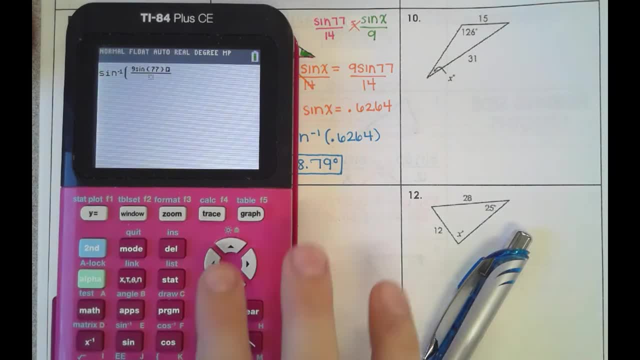 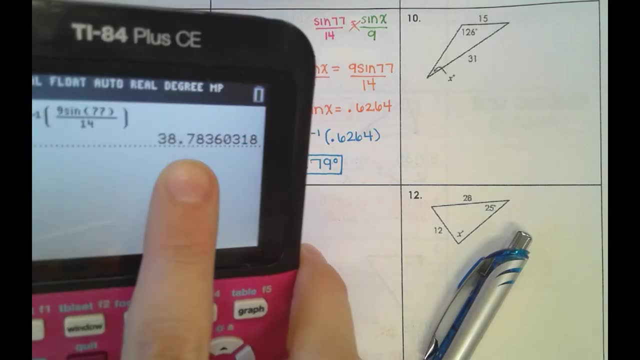 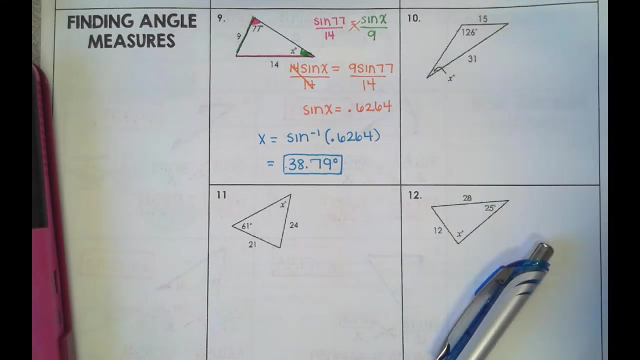 nine sine of 77 over 14. I mean it was off. you know it's really should probably be seven, eight, because we ran, we round it up a little bit here, so it made this round up. so if you want to completely skip turning it into a decimal, you can all right. so number 10: 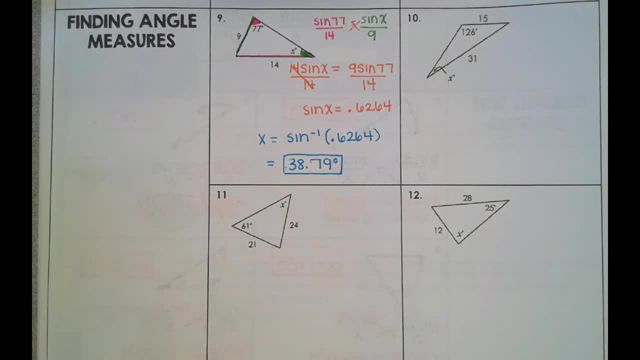 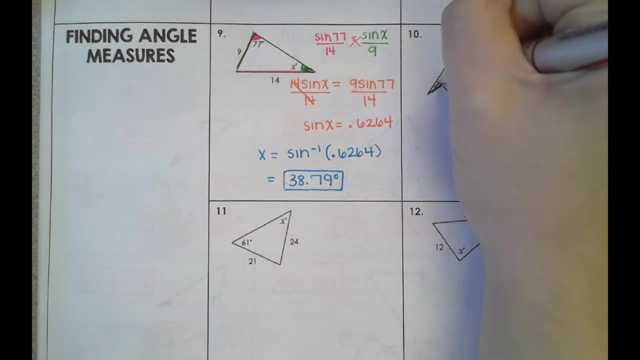 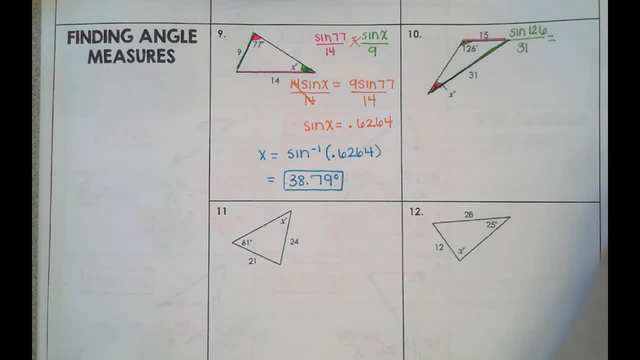 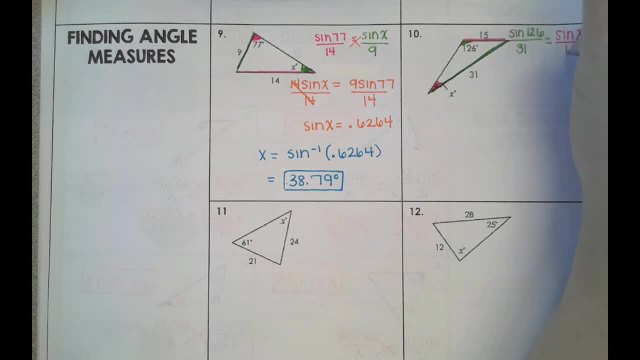 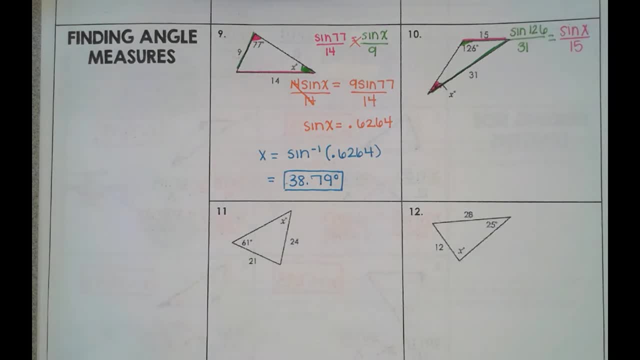 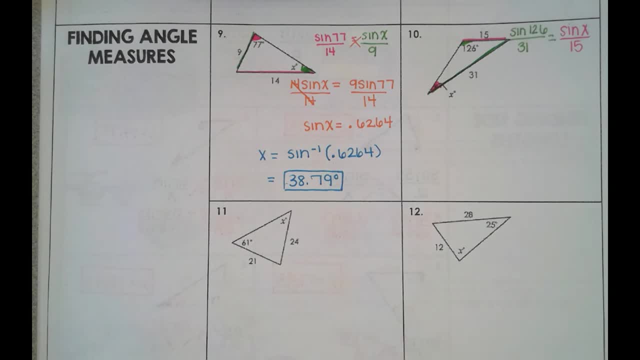 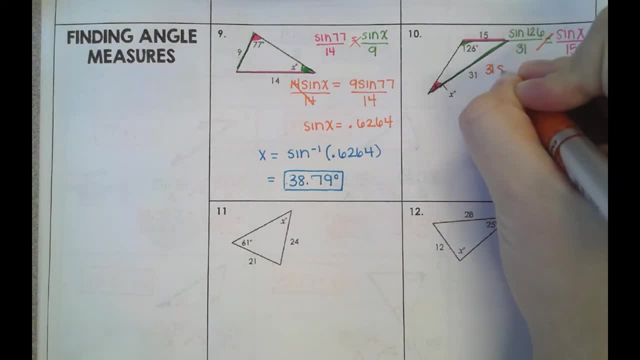 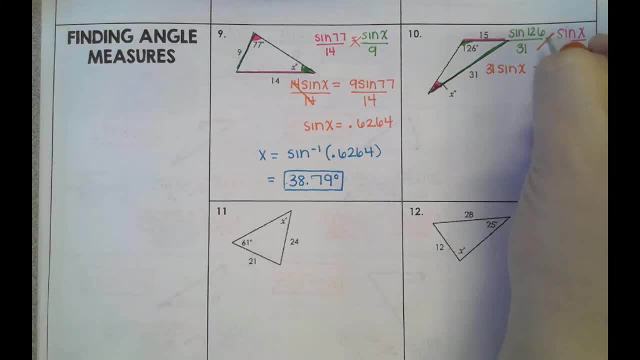 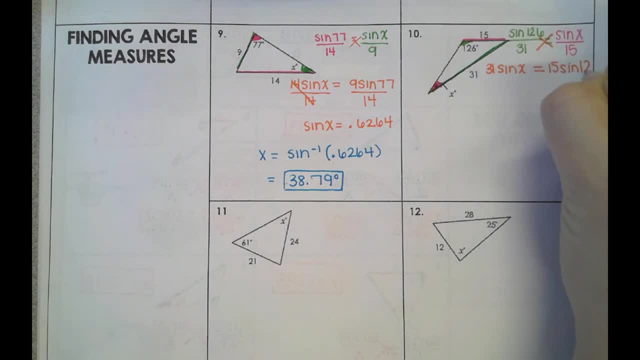 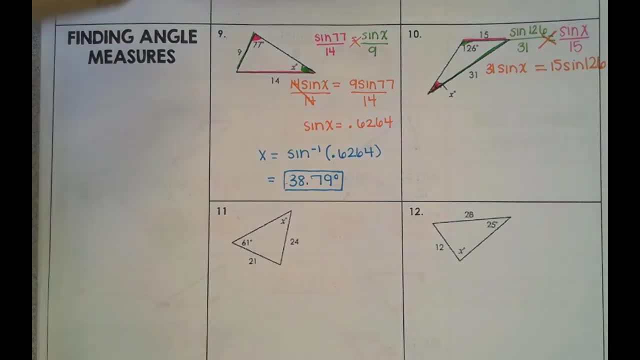 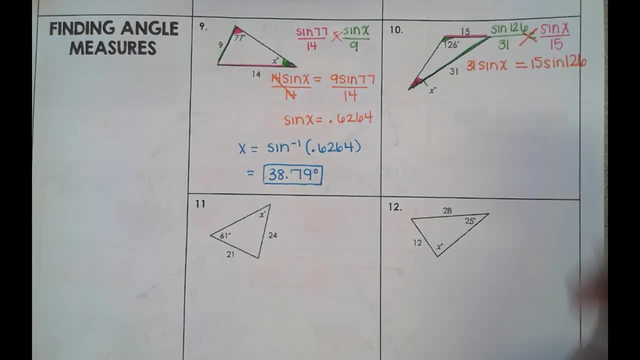 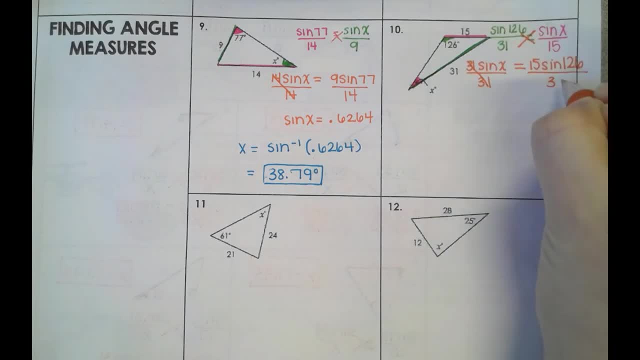 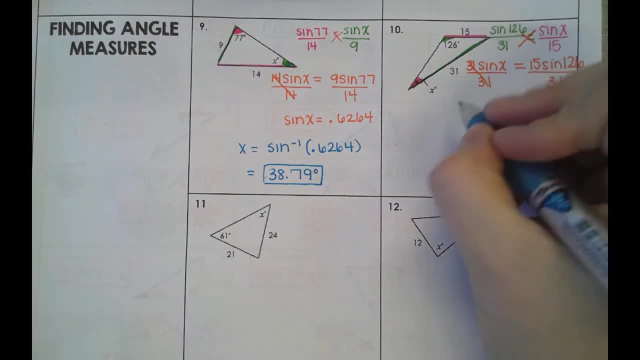 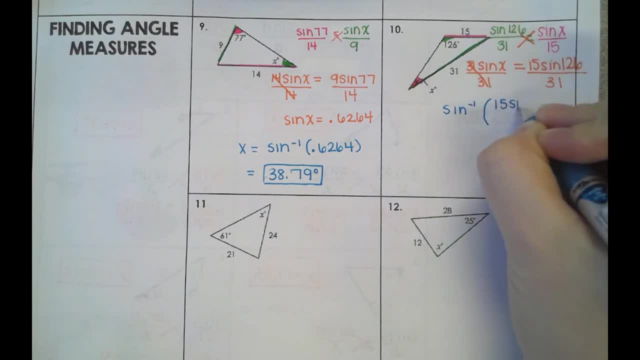 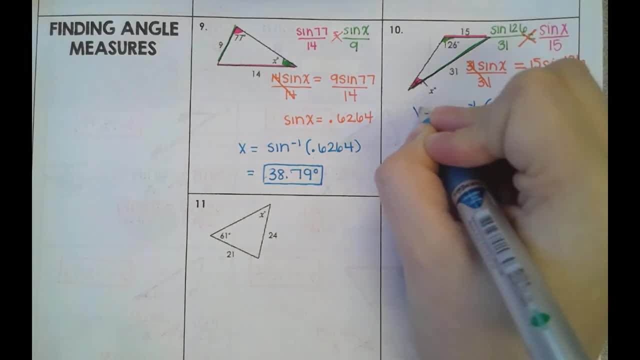 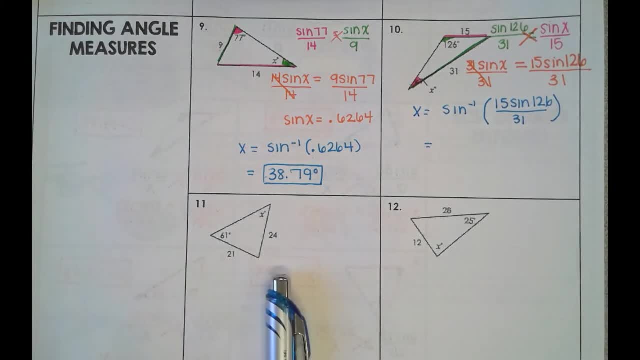 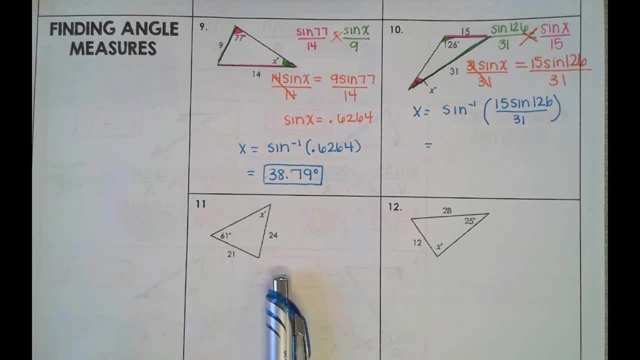 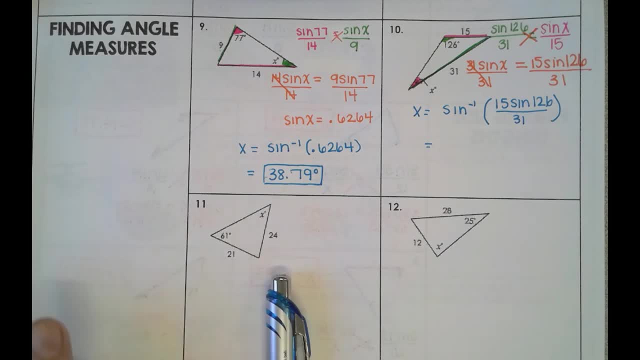 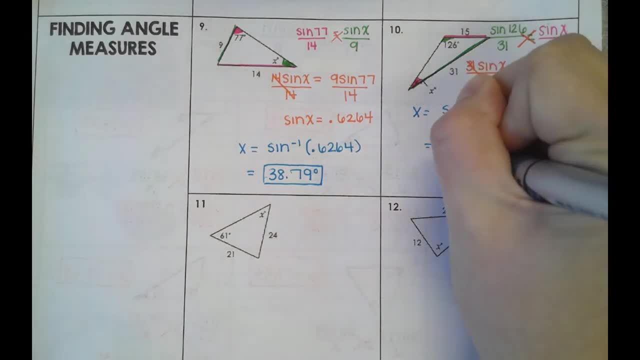 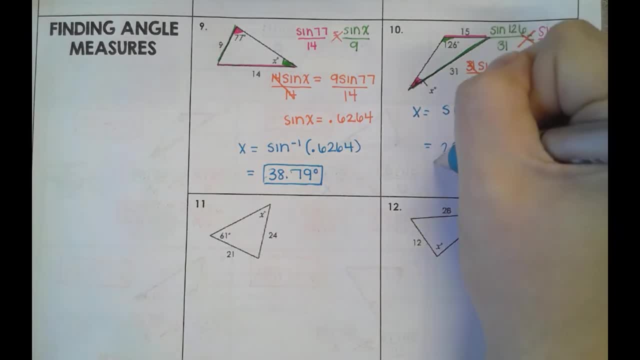 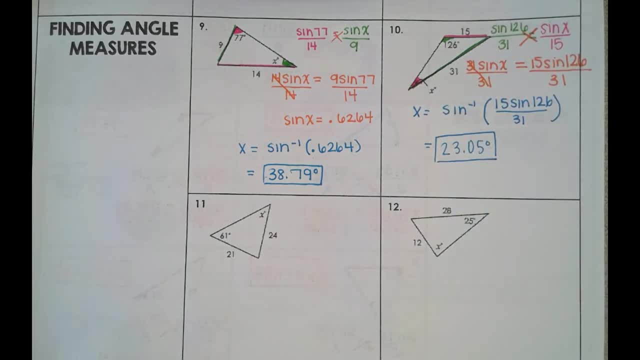 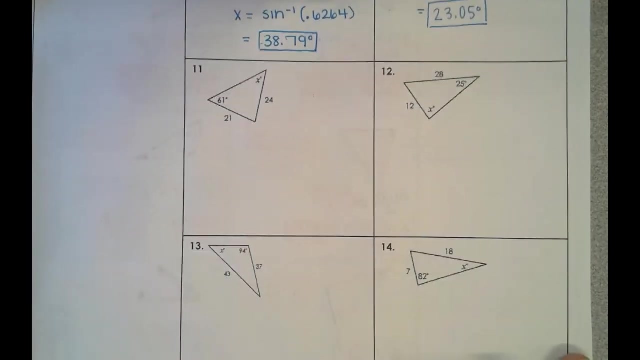 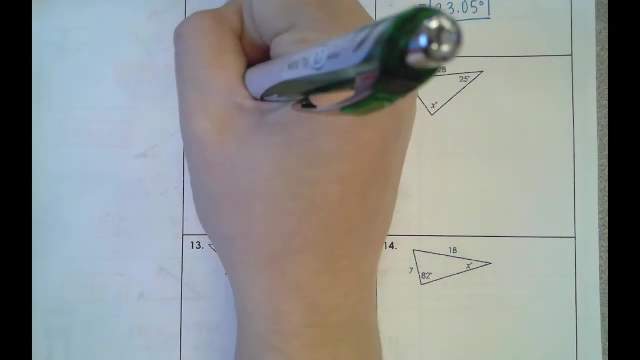 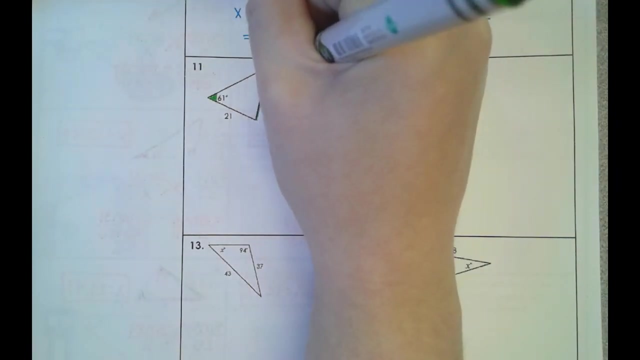 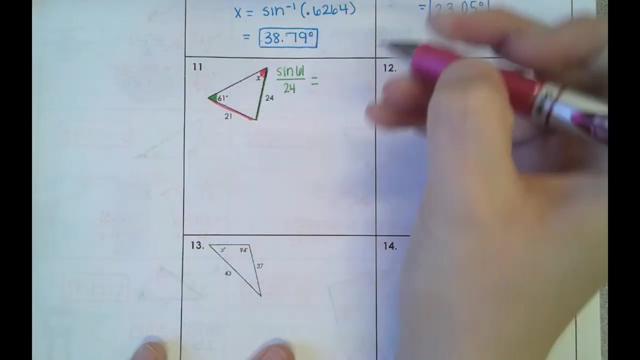 And you should get about 23.05 or so. Any questions? A couple more? All right, so 61 degrees matches with the side length of 24.. So sine of 61 over 24 equals sine of x over 21..